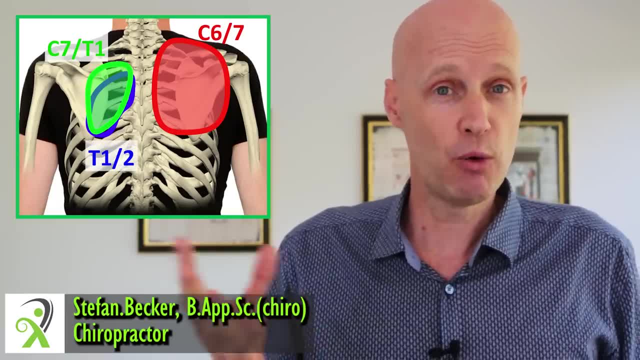 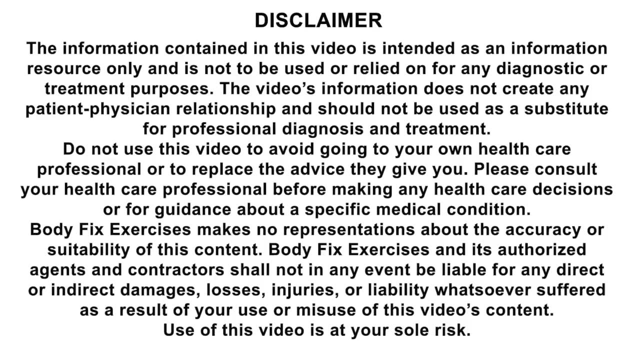 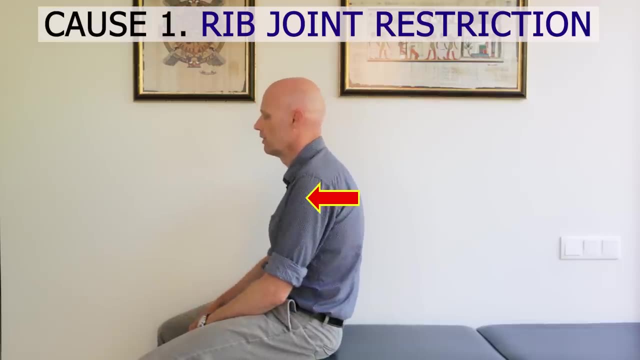 So in this video, I'm going to show you how to get rid of this type of pain quickly with a few exercises and how to avoid it coming back When we slouch with a rounded back or lay on one side with our shoulder pushed forward. 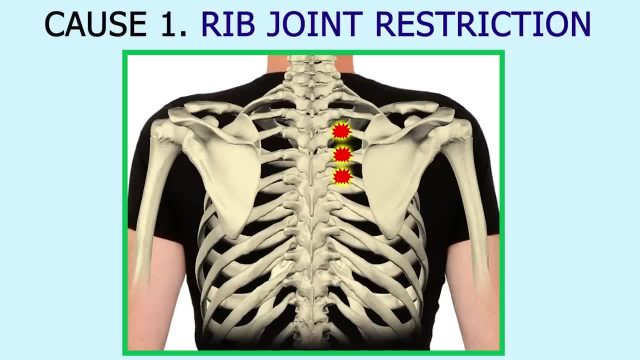 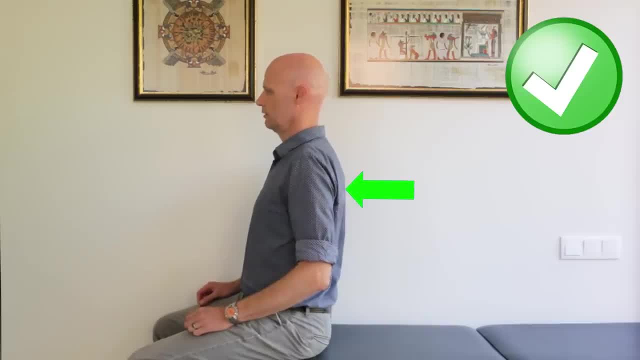 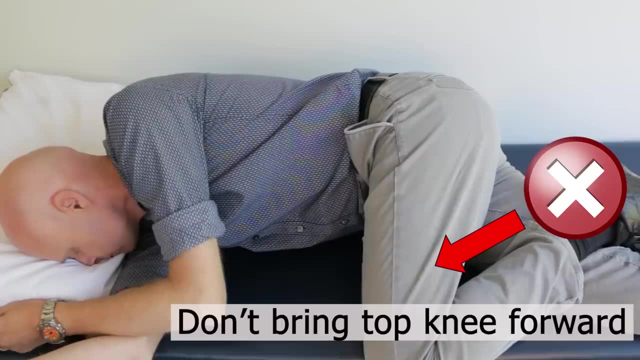 it can jam the joints between our ribs and the spine, causing pain and muscle tightness over those rib joints. So try to be more aware of your sitting position and, if you're a side sleeper, avoid rolling forward, as this will push the bottom shoulder forward and distort the rib. 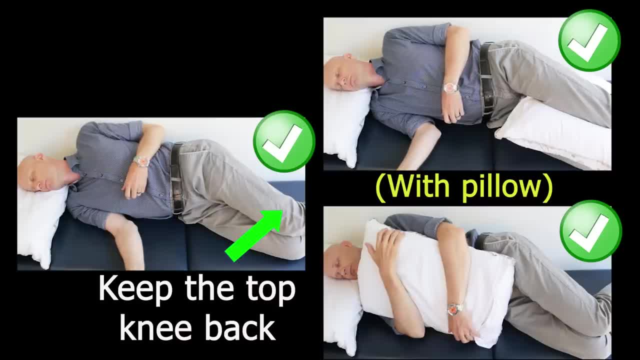 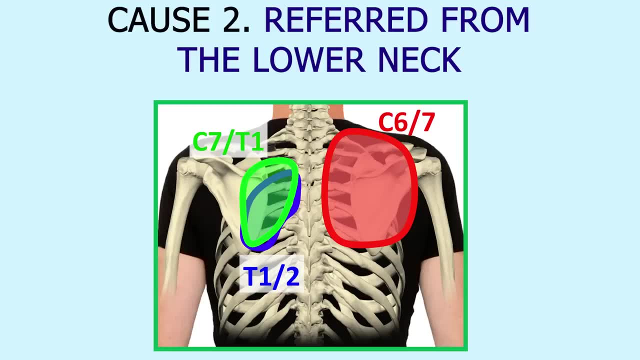 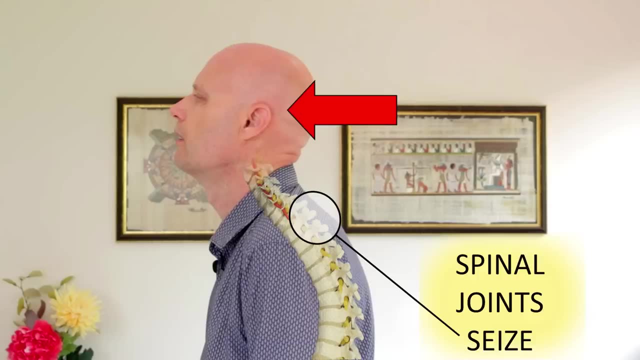 cage. Keeping both legs bent evenly when lying on your side can help to avoid this position. The other cause of pain in this area is referred pain from the spinal joints at the base of the neck. The spinal joints get jammed and irritated from forward head posture or looking down at. 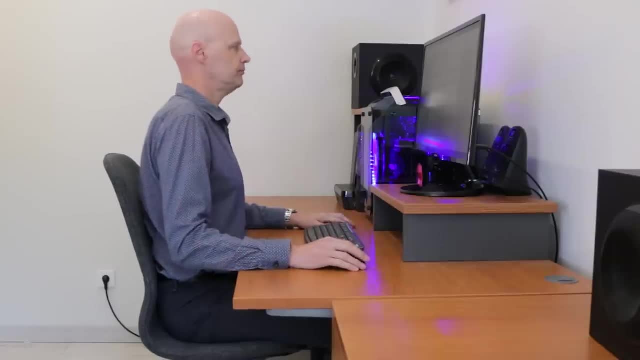 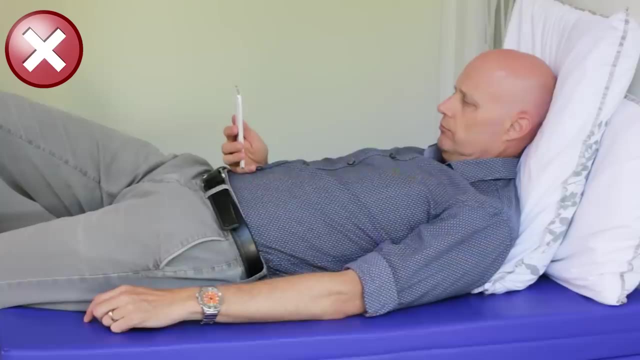 mobile phones and laptops. So keep your chin back when you're at your desk. lift computer screens and keep your mobile phone up, and avoid sitting in bed or on the couch with gadgets positioned on the back of your head. So keep your chin back when you're at your desk. lift computer screens. 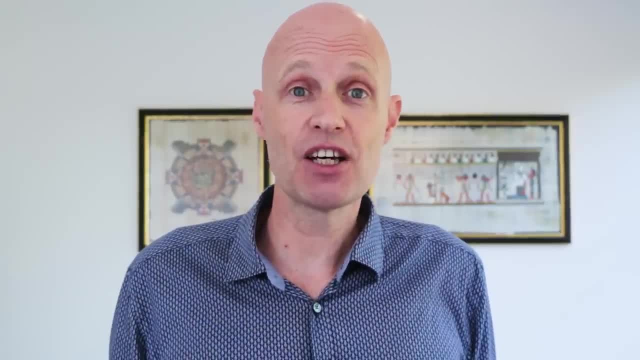 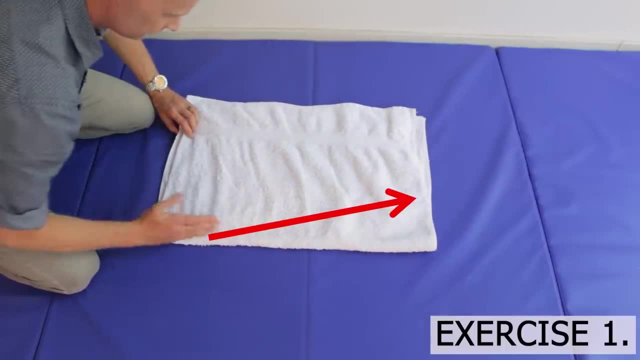 and keep your mobile phone up, and avoid sitting in bed or on the couch with gadgets positioned on your stomach. Fortunately, there's five great exercises that work on both of these issues, and they only take about a minute each Exercise. one: Roll up a towel on a slight 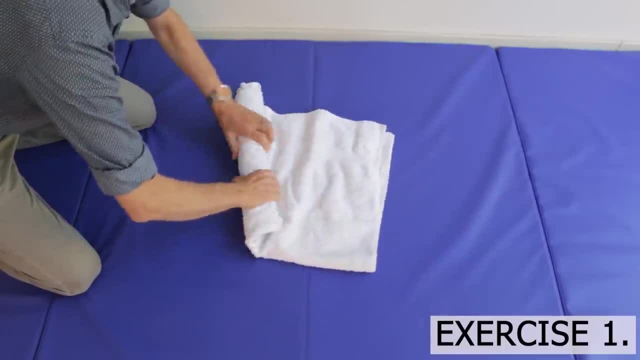 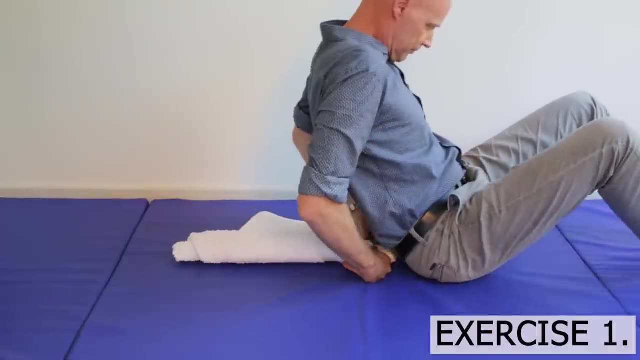 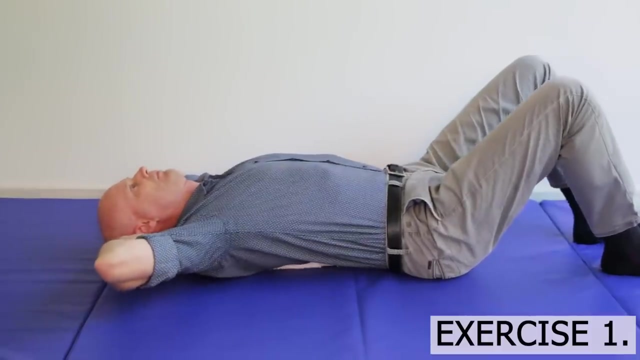 angle to create a towel roll that's about 10 centimetres thick- that's the length of your mid-back- and slightly tapered at each end. Lay down on the roll on the floor, not a bed. Make sure you bend your legs and put your hands behind your head. Start off. 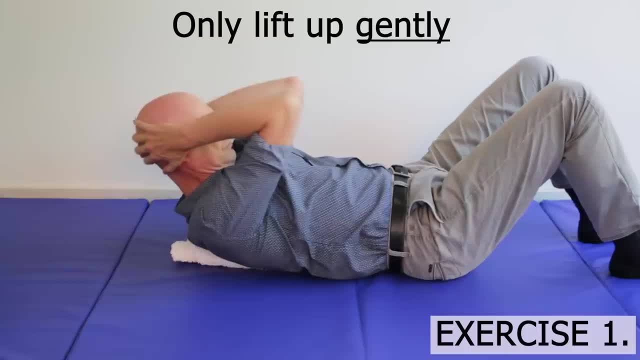 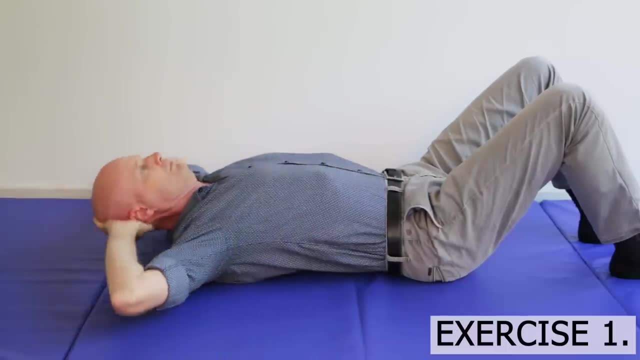 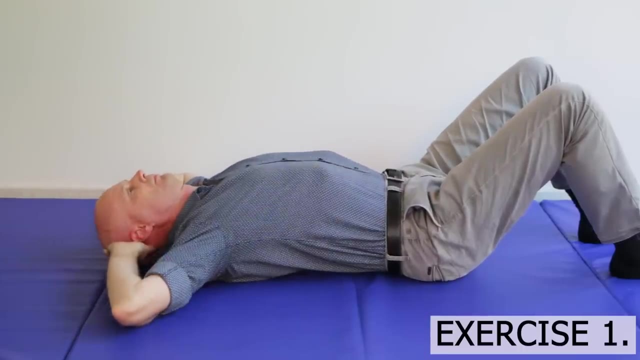 by gently lifting your elbows and head and then lowering them several times to mobilize the rib joints and the thoracic spine. You may hear some mid-back or rib joints release, but that's fine. Then just lay there for one minute to stretch the rib joints back and 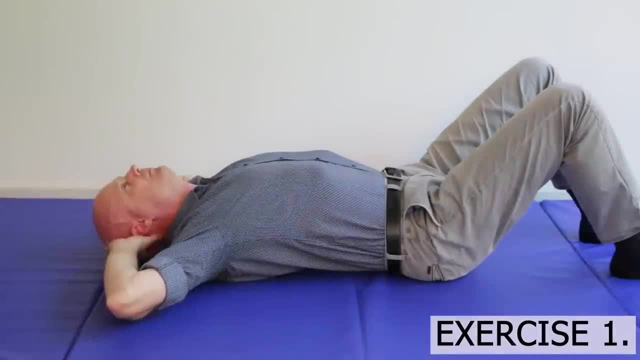 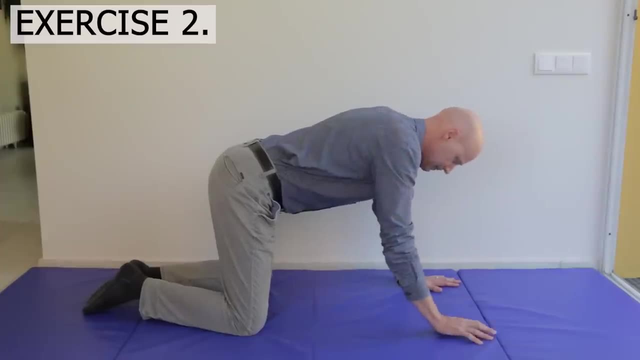 to open up the lower neck joints. Make sure you're looking up, not back, to ensure that you have your neck in the best position. Exercise two: Now let's mobilize the rib joints joints and the lower neck joints with some rotation On your hands and knees. 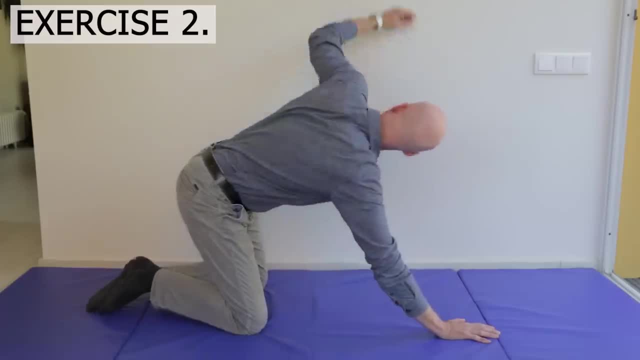 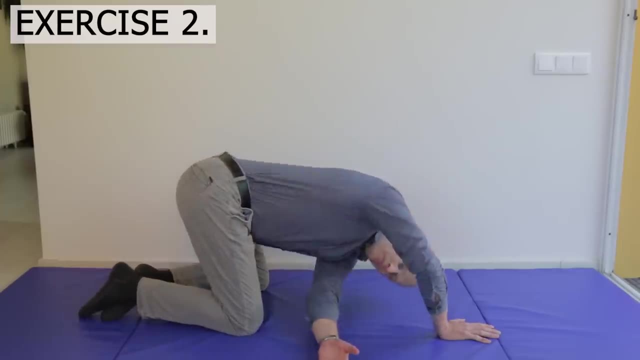 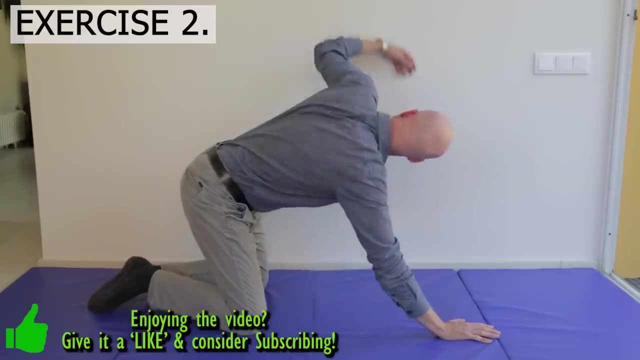 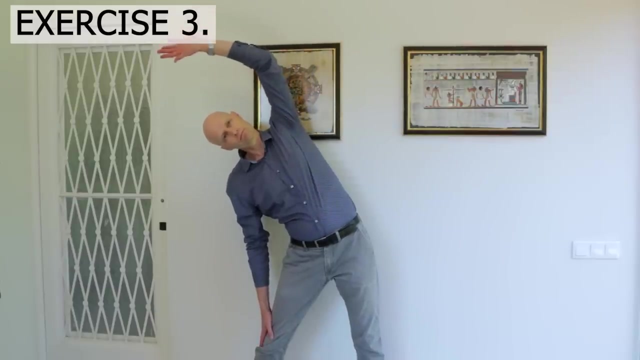 reach up with your hand towards the ceiling and look in the same direction, Then reach through to the other side underneath your opposite arm. Keep moving slowly rather than holding these positions, and repeat five to ten times each side. In exercise three, we move the ribs and lower neck into the third plane. 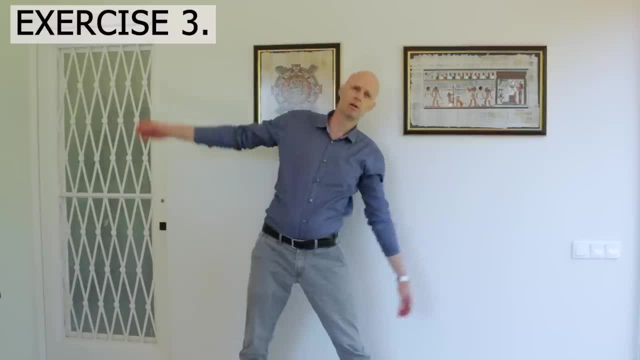 of motion: side bending, Standing. bend your arms, head and torso from one side to the other, slowly keeping them all in a line Again. you may hear some rib joints release as they start to move more again, but that's pretty normal. Repeat ten times. 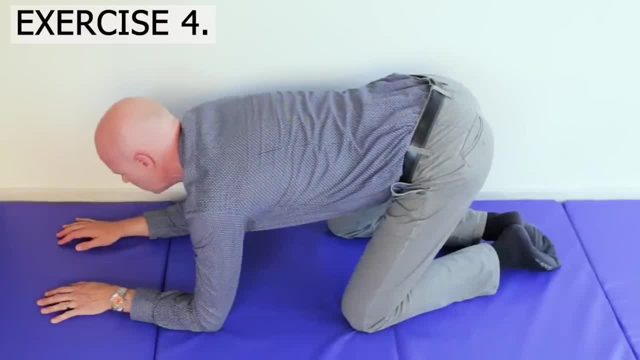 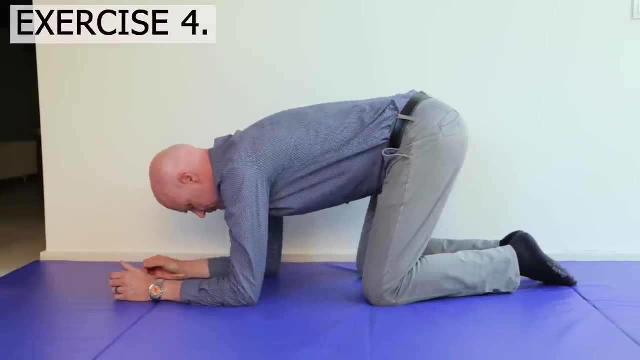 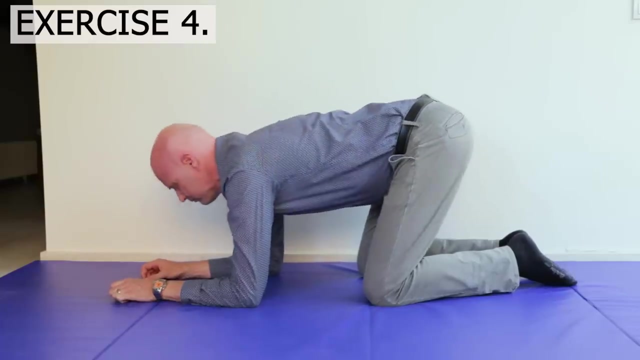 slowly Exercise four. Next is a thoracic cat cow, but with a specific neck position. Begin on your knees and elbows, with the pelvis slightly behind the knees, and then alternate between a protruded and extended mid-back position. The neck goes in the opposite direction. 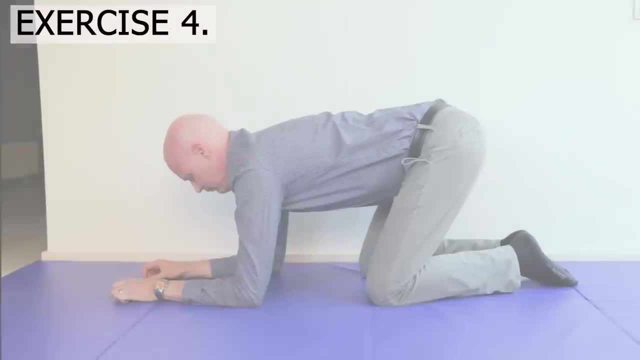 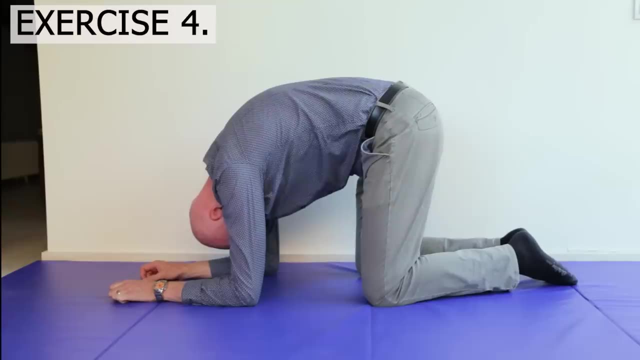 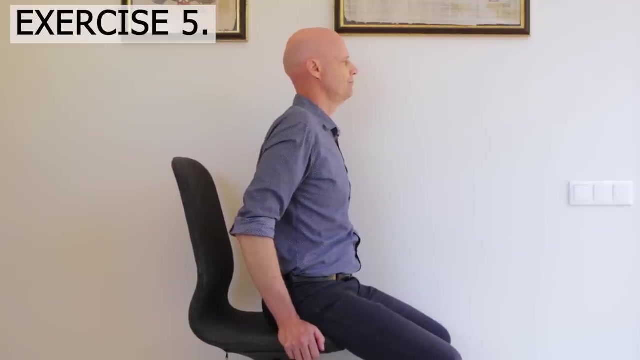 to the thoracic spine, but when you bring it back, keep the chin tucked in to open up the lower neck joints. Repeat ten times slowly, Exercise five. The final exercise is a chin tuck plus Sitting with your hands on the floor. with your hands on the floor, with your hands on the floor. 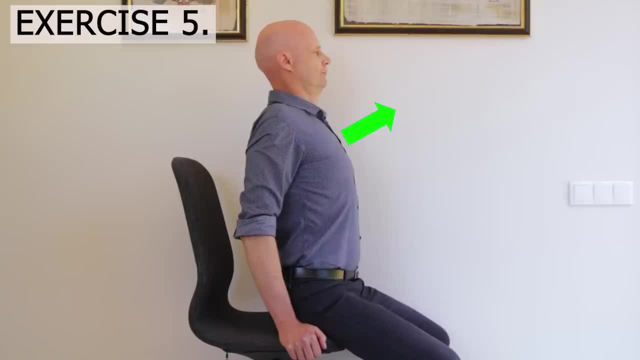 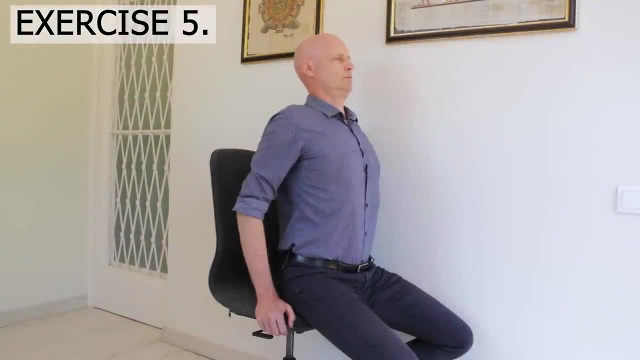 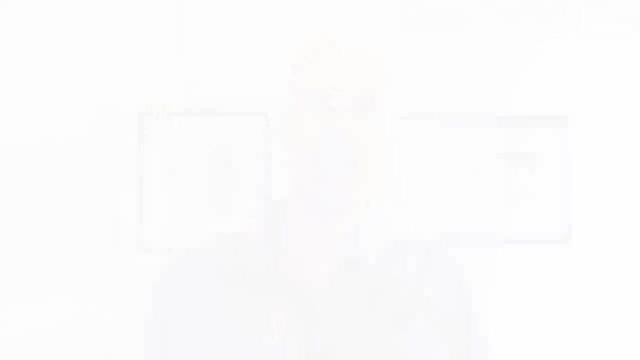 with your hands each side of your hips, protrude the chest to extend the mid-back and then retract your neck straight back, keeping your chin down. This will open compressed neck joints and mobilize the upper thoracic area. Repeat ten times, slowly. Anyway, that's it for today. I hope you liked the video. If you did, please. 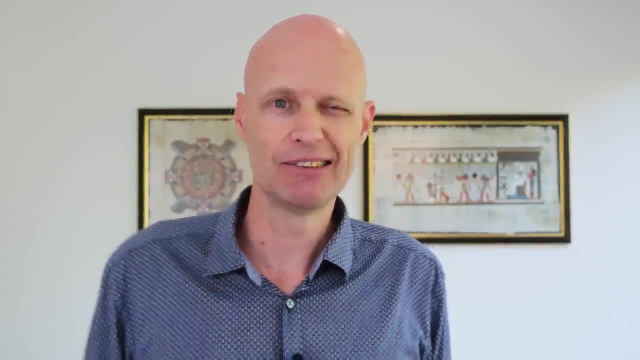 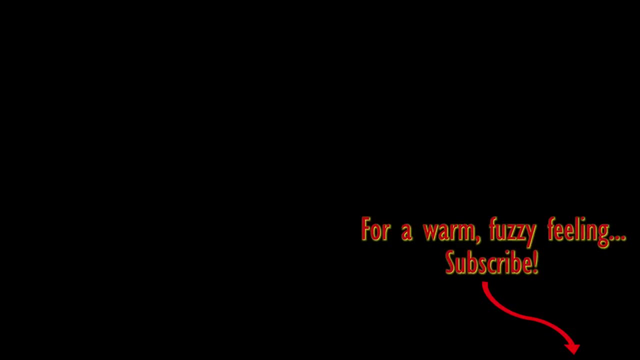 consider liking, commenting and subscribing, because it really helps. Okay, cheers. So in this video, I'm going to show you the fit that did you become. Thank you for watching and I'll see you in the next one.